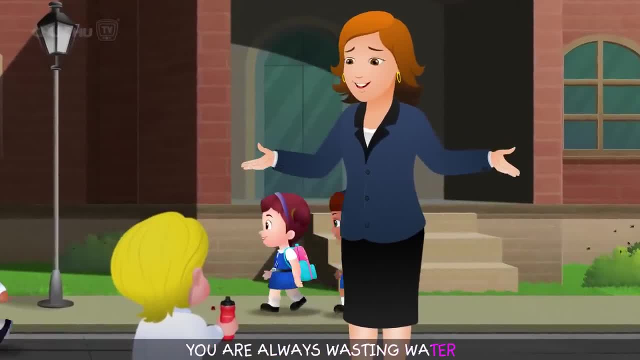 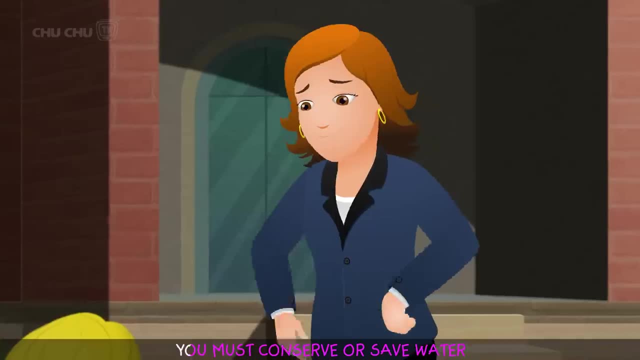 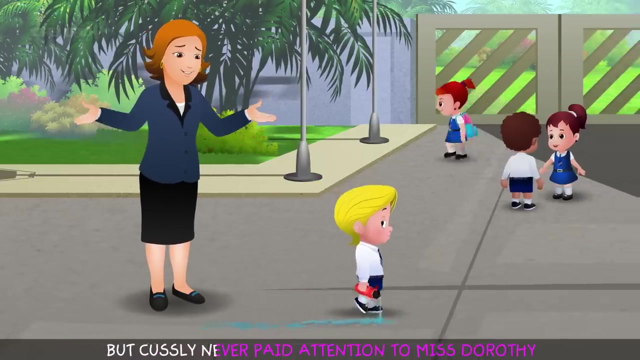 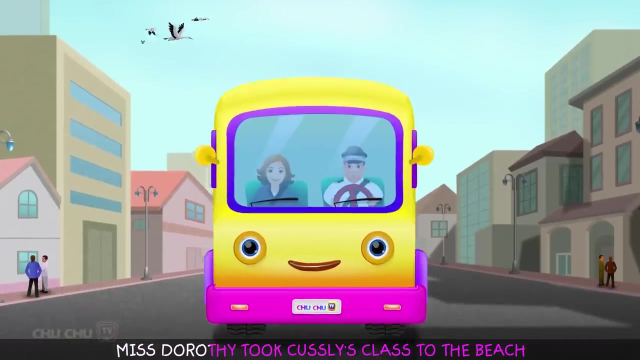 Custly, you are always wasting water. You mustn't do that. Water is very precious. You must conserve or save water. But Custly never paid attention to Miss Dorothy. One day Miss Dorothy took Custly's class to the beach. 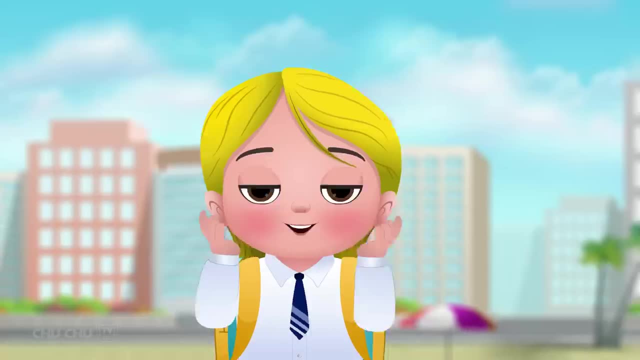 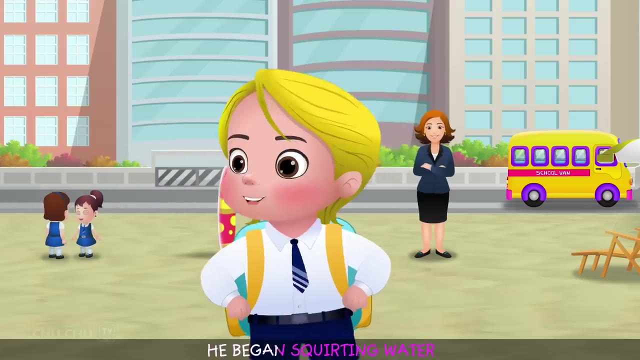 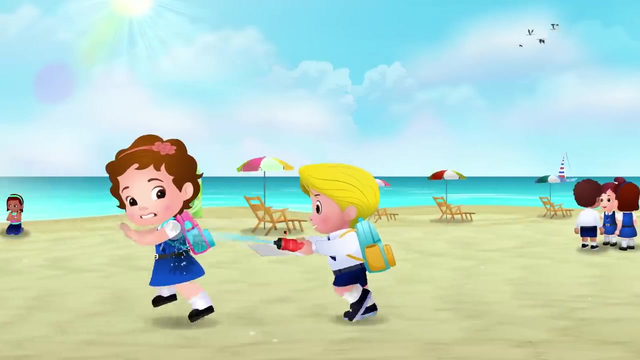 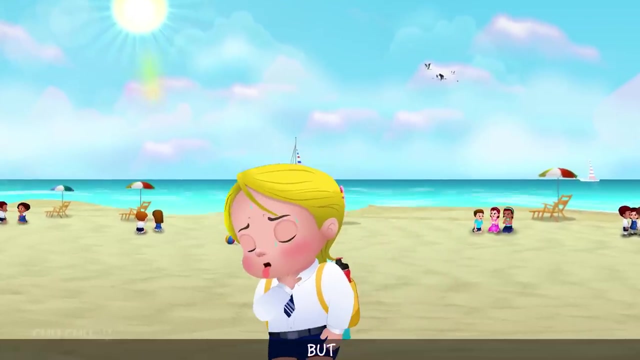 It was quite hot and sunny there, Custly, you are always wasting water. Custly wanted to have fun, And so he began squirting water from his water bottle everywhere. After some time, Custly felt thirsty, But when he opened his bottle to drink some water, 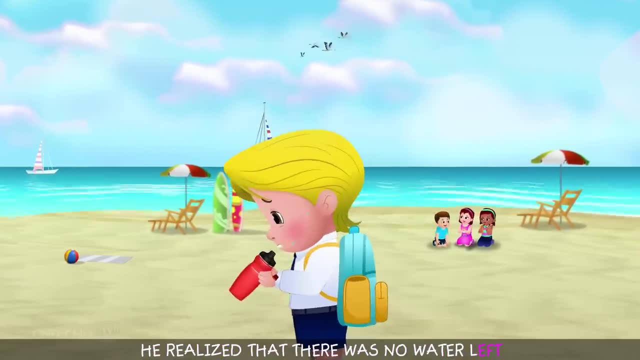 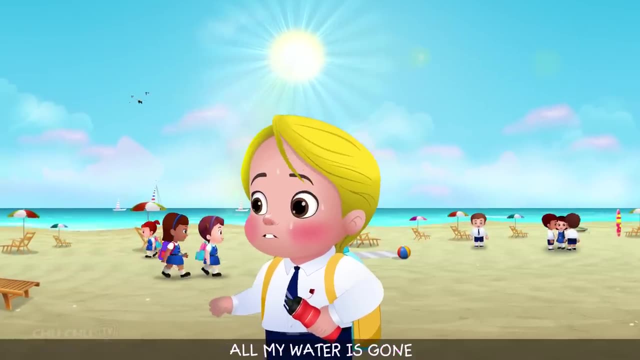 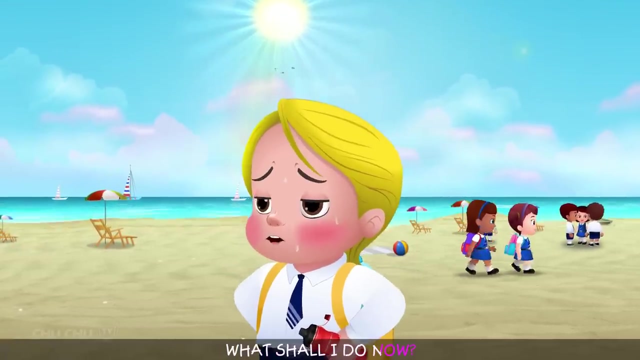 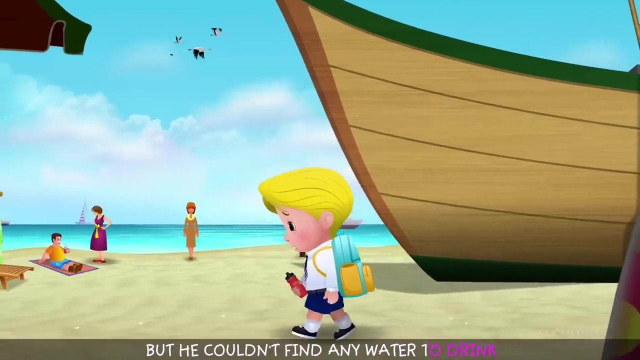 he realized that there was no water left. Huh, Oh, my water is gone And I'm very thirsty. What shall I do now? Custly looked all over the beach, But he couldn't find any water to drink. Oh, my throat hurts. 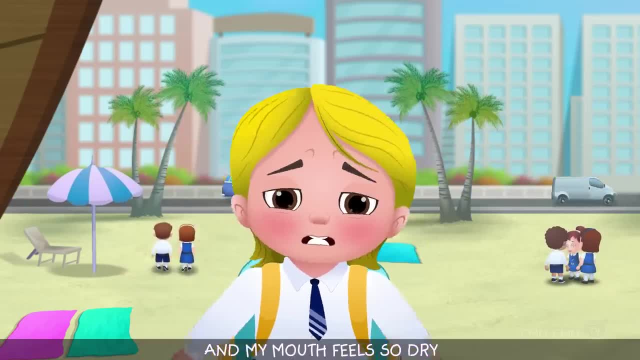 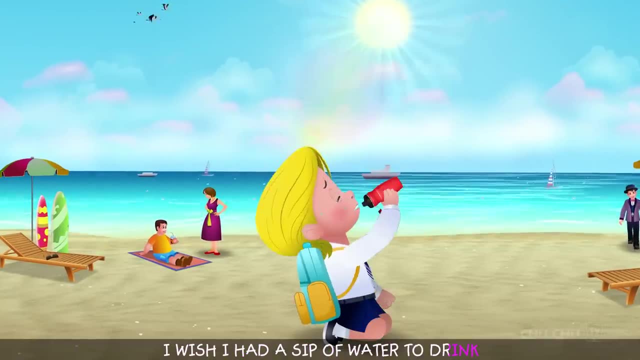 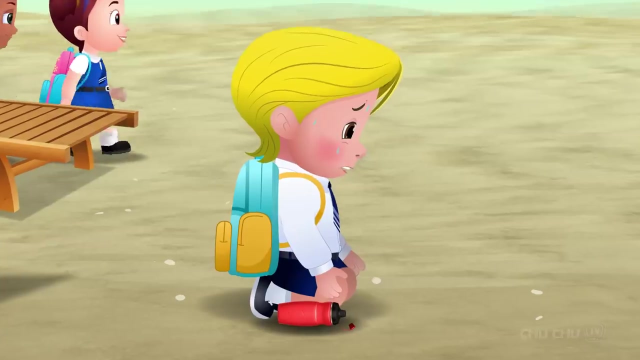 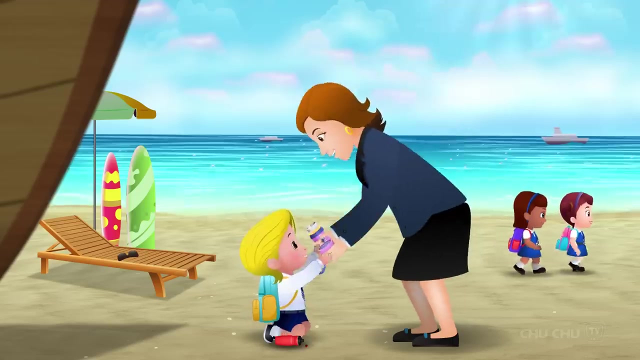 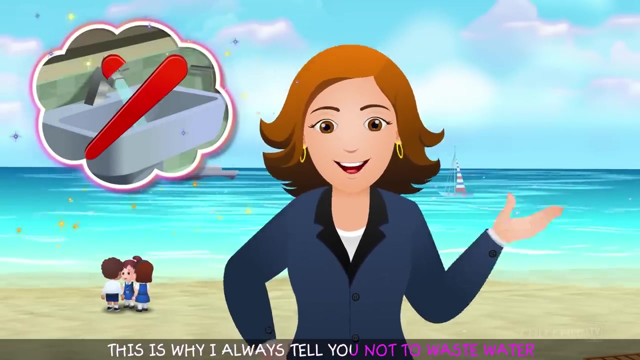 And my mouth feels so dry. Hey, I wish I hadn't wasted the water I had. I wish I had a sip of water to drink. Miss Dorothy noticed Custly. She gave him some water from her own water bottle, Custly. this is why I always tell you not to waste water. 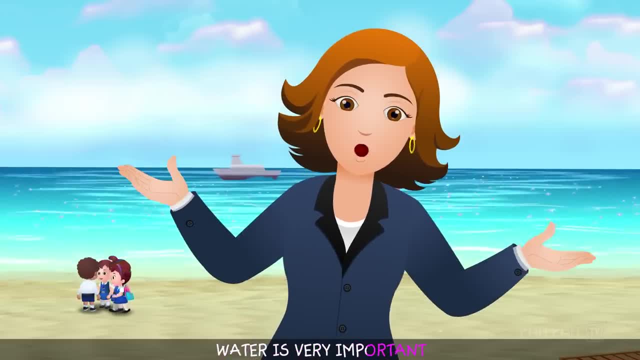 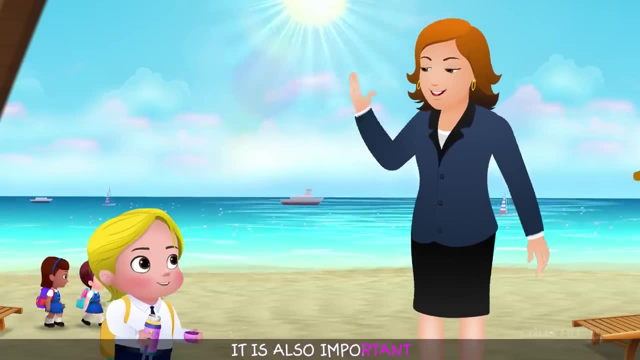 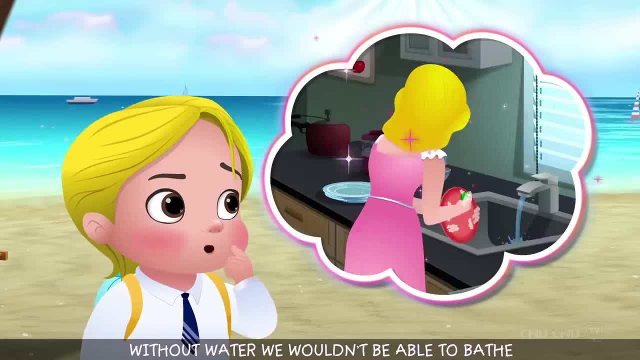 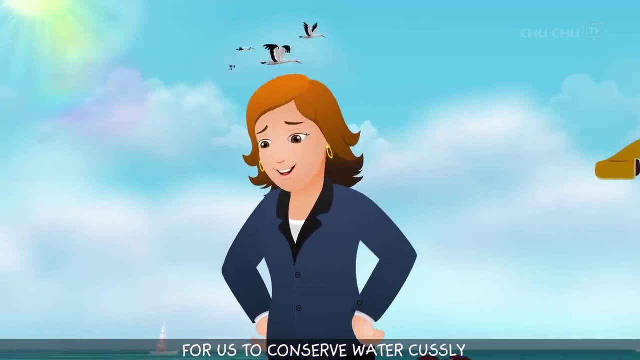 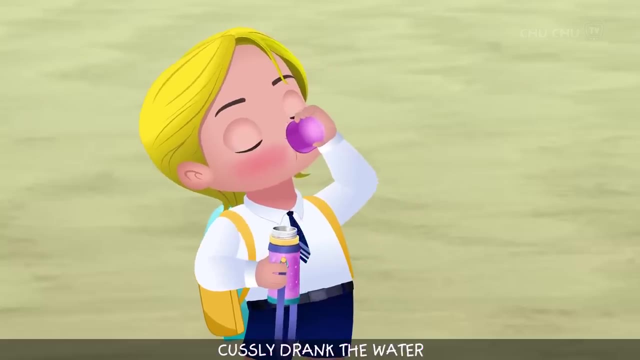 Without water, we wouldn't be able to bathe, clean or survive. That's why it's important for us to conserve water Custly. We must save every drop we can. We must save every drop we can Custly, drank the water and thanked Miss Dorothy.